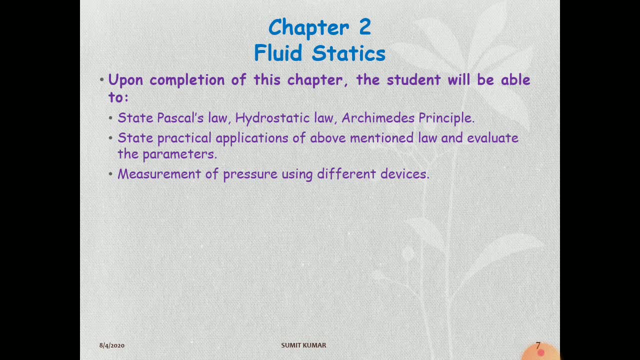 Hydrostatic force, center of pressure, buoyancy, stability of submerge and floating body in fluid will be discussed.